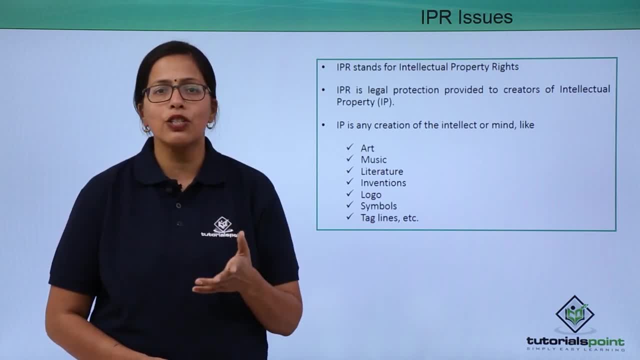 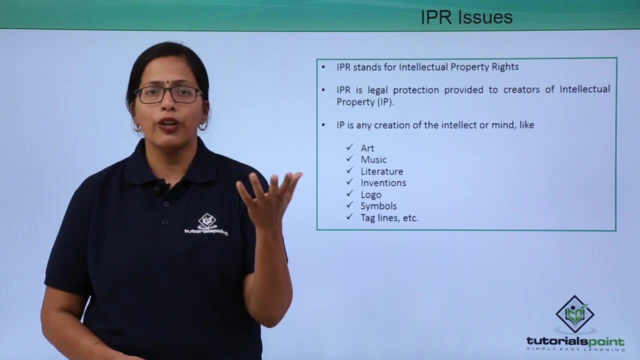 creation of the mind. What do you understand by any creations of the mind? So any art piece that you have created, any music that you have created, any literature, poetry, fiction, non-fiction that you have written, any inventions you have done, scientific inventions. 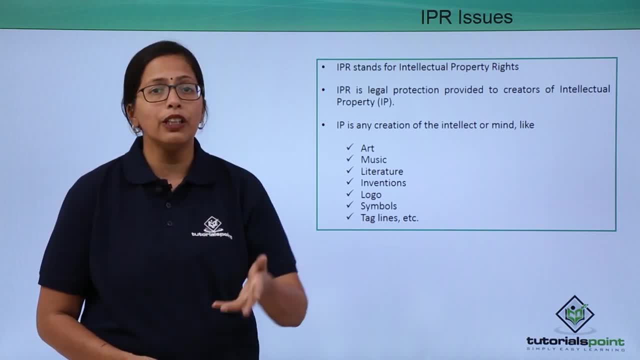 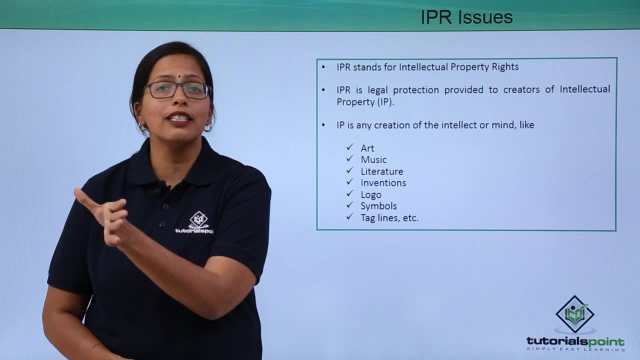 any logos that you have created, you have designed for your company or anyone else, any symbols that you have come up with, any taglines. all the companies are having a taglines associated with them, So that also comes under the intellectual property. 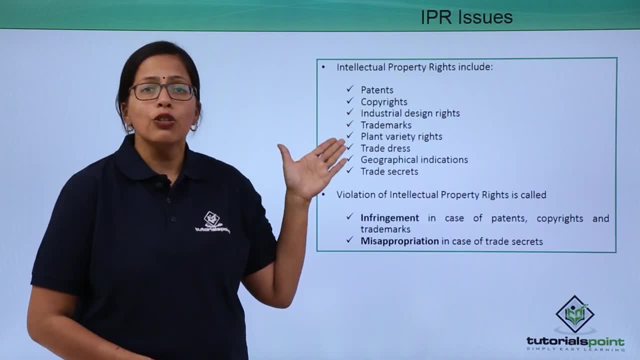 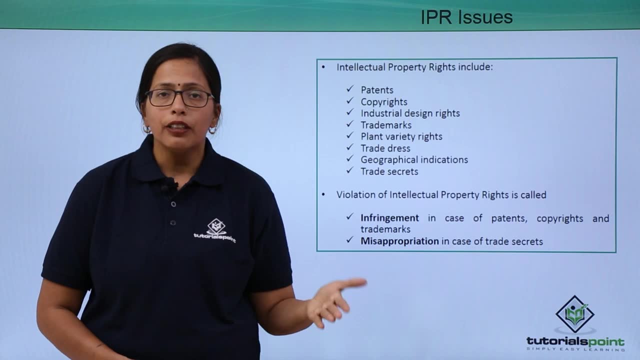 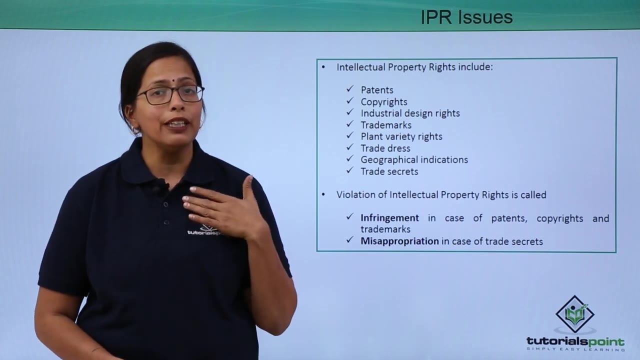 Intellectual property rights. Intellectual property rights will include the patents, So any creation of art, music, literature, logo, symbols. if I have created them, then I hold a right to it. That means that nobody can use it, nobody can reproduce it without my permission. These rights cover. 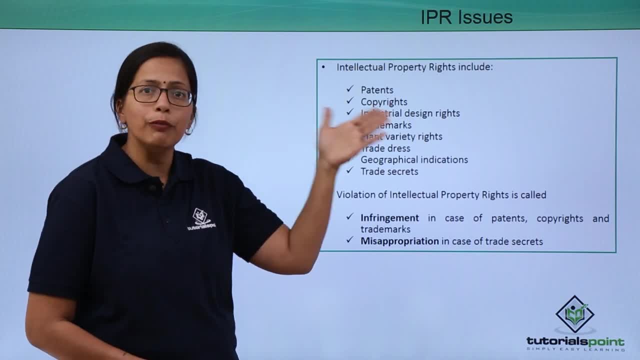 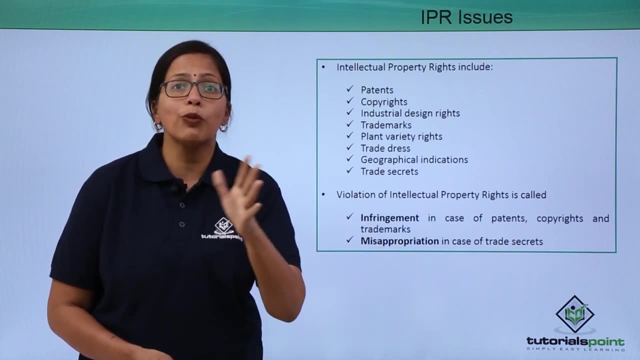 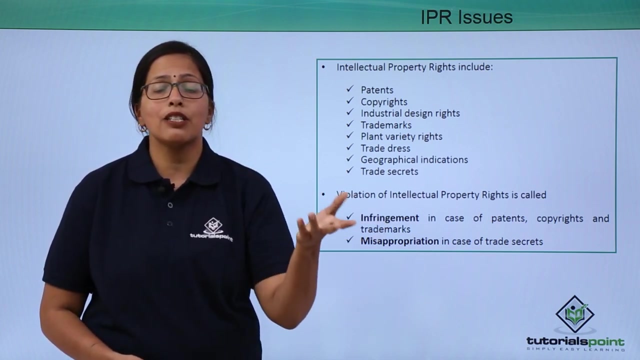 patents, copyrights, copyrights for my music, for my literature. industrial design rights: that means some design, some industrial design, some automobile design that I have created. Plant variety rights- If some new plant varieties of, say, maize or rice or mango have been created by the scientists, developed by the scientists. 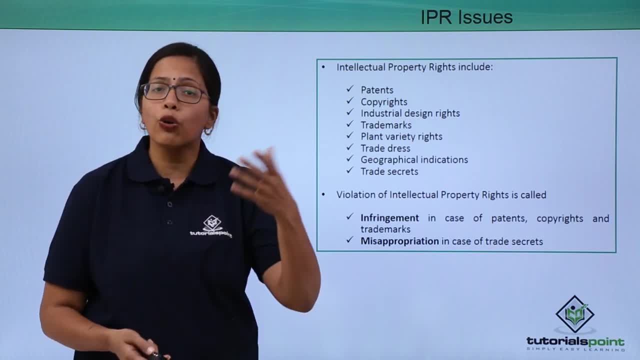 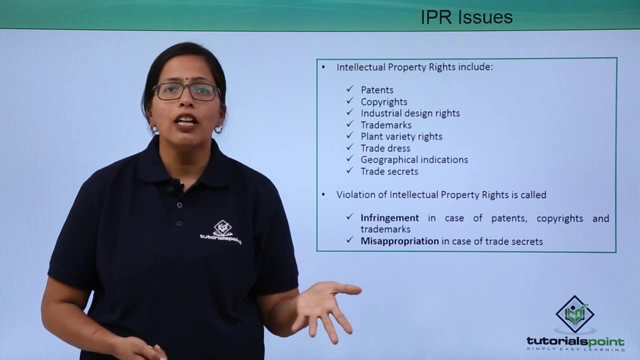 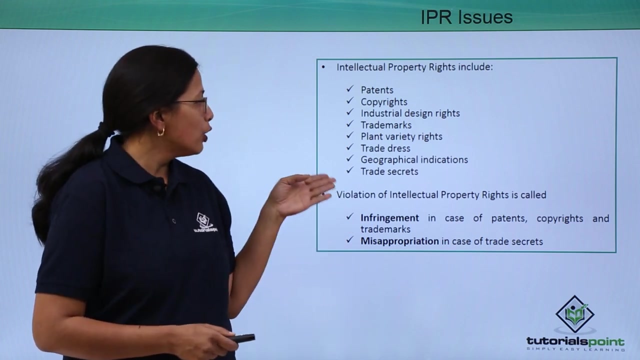 then they hold a right to it. No one can grow these crops without their permission. Trade dress: If any company, any organization has designed a dress specifically for their employees, then they hold a copyright to it. Then this is the commercial corporation here. the people who own this property don't need to pay. 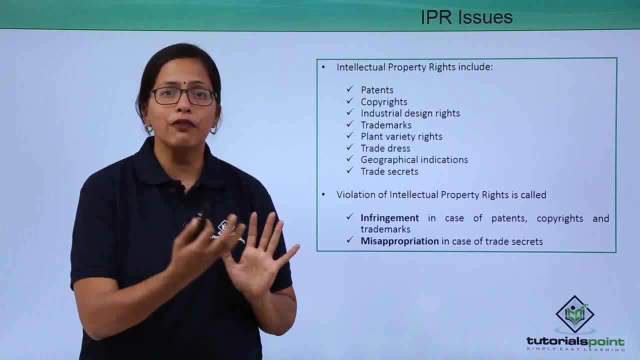 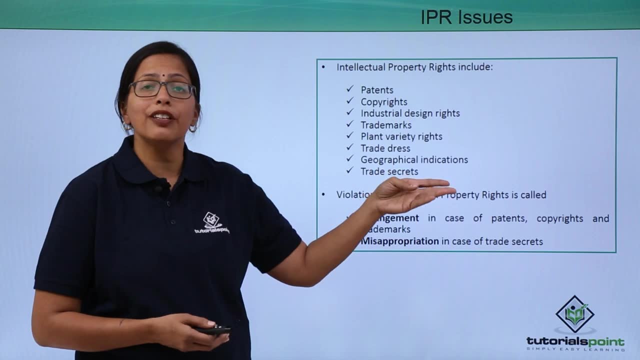 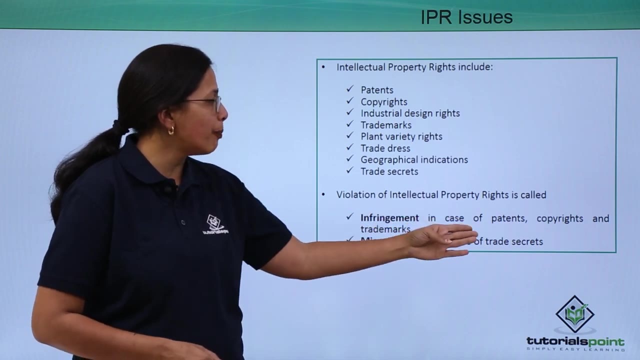 tax, They can also take the property right. They are not too surprised if in public institutions there are some いうこと on data points, on trade secrets往u huир rãghācāt ki ex Yao vai āpākākāyārā案 yudween yā. These clients who own these workersftbull komenaiña costs, economic audit center, funds, transfer funds go to the Point Denominator for money releasing. So they don't come to mind that some ways that they will do things Go to the point in front of you and they will take away the rights, say like if they backwards into the Republic of India and they leave the Generation Supt unveiling the Pages in the future, then the money will come right away. Styles Turn back to face to face Now that because in particular, these lawsuits in the volunteerakanat